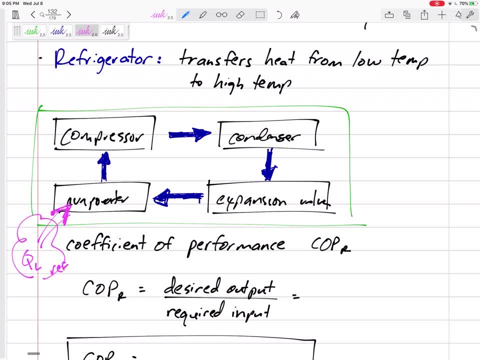 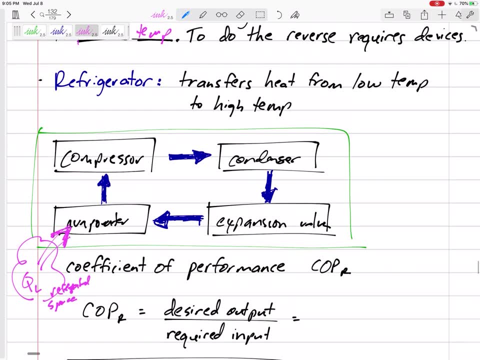 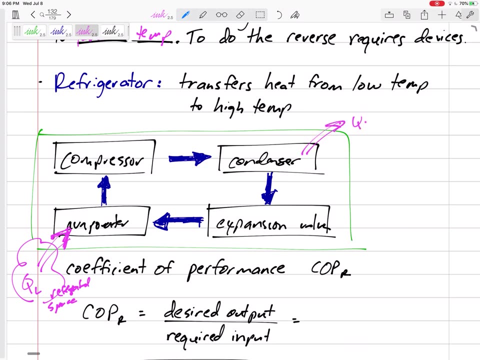 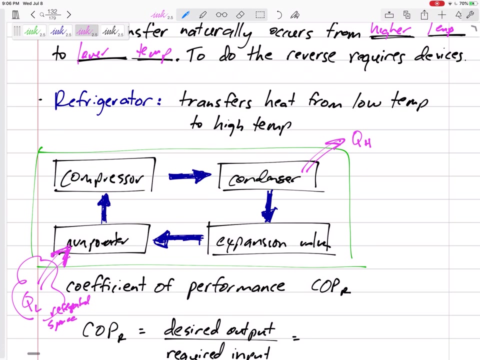 from the refrigerator, Refrigerated space, refrigerated space and it expels some heat. QH to the behind the refrigerator. Okay, refrigerators, don't really throw cold air on your, on the food and the drinks and stuff in the refrigerator. It really takes away heat. It takes away heat from the refrigerated space. 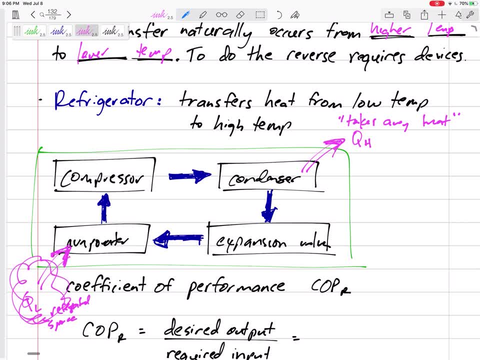 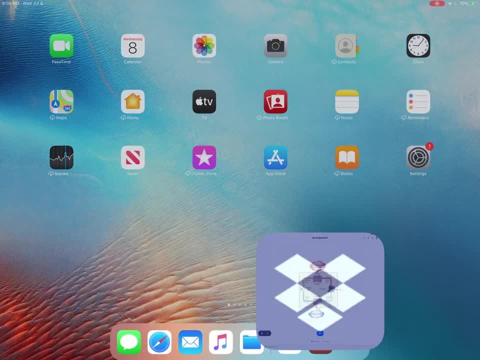 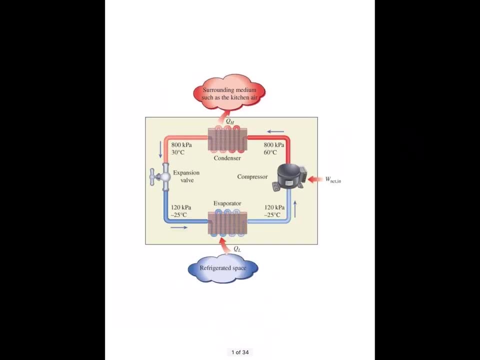 It takes some of that QL and it spits out the QH outside behind the refrigerator. Look at the. the book does a better job. Look at the book's figures. This would be a refrigerator This down here. you can't see my. 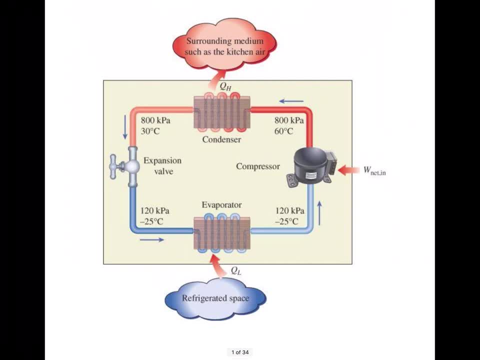 this down here where the QL is, that is the refrigerated space. But then inside the refrigerator there's evaporator, compressor, condenser, expansion valve and there is refrigerant going through here And the refrigerant accepts that QL, The refrigerant goes to the compressor. It 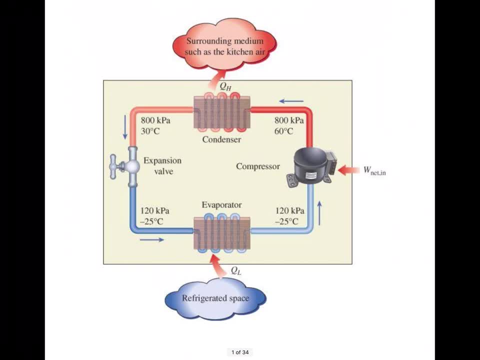 needs some work. That compressor needs some work. It heats up, Then it goes through condenser and it spits out that QL out the surrounding medium, Out out the back of the refrigerator. All right, if you ever notice that it is. 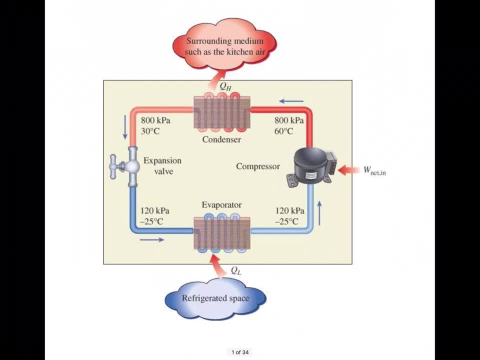 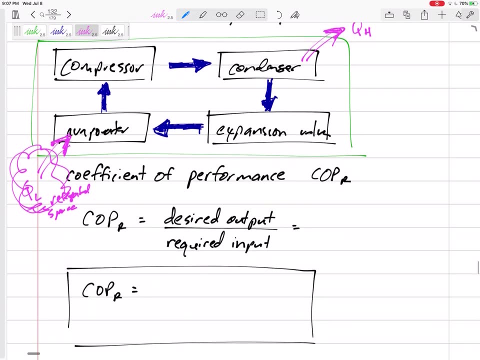 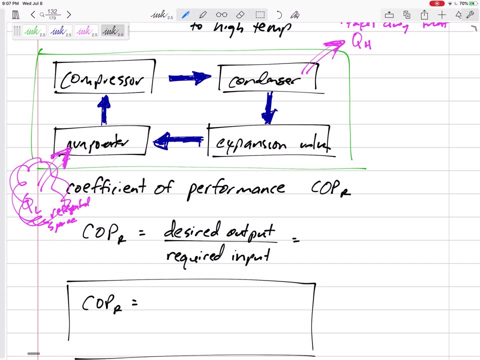 hotter behind your refrigerator because it's expelling that Q QH. Okay, so instead of efficiencies, instead of efficiencies of refrigerators, we have the COPs, the coefficient of performance of a refrigerator. So the coefficient of performance is the desired output over the required input. So, for a refrigerator, what are you really? 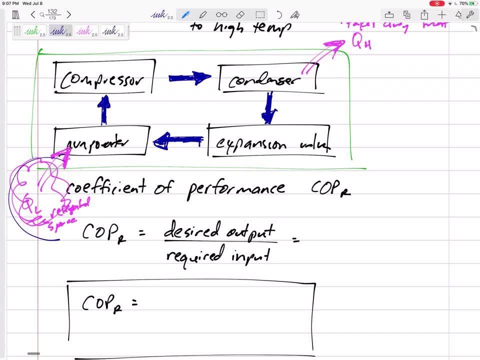 the goal of the refrigerator. The goal of the refrigerator is to take as much heat away from the food and drinks as possible. The QL: we want to get as much QL as we can. So the QL is our desired output. The required input would be over here. I've got this backwards, I think. 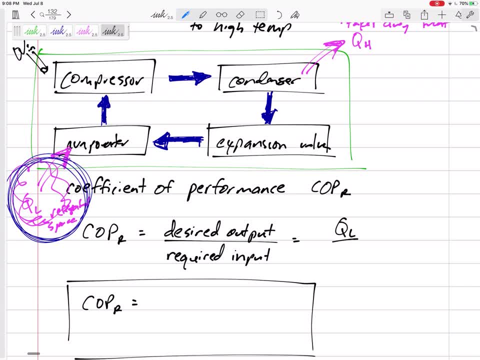 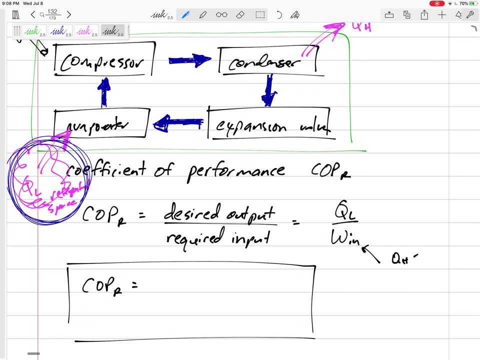 the compressor. uh, the work in the required input is the work in. all right, we work in is q h minus q l right here, all right. so the coefficient performance of a refrigerator is q l over q h minus q l. or if we divide all three of those by q l, we've got one over q h over q l. 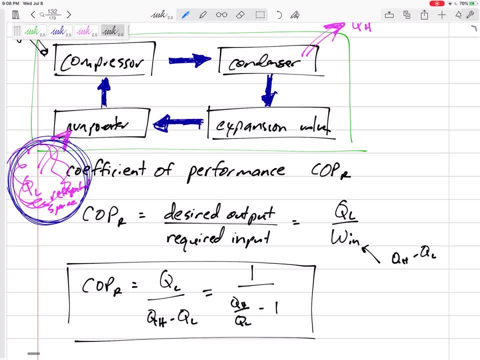 minus one. so all right. so that's the coefficient performance of the refrigerator. it can be greater than one, so it's not like efficiency that has to be less than one. it definitely can be greater than one, but it doesn't mean it's it's um emitism. 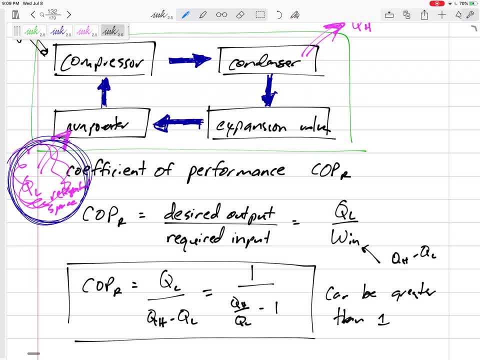 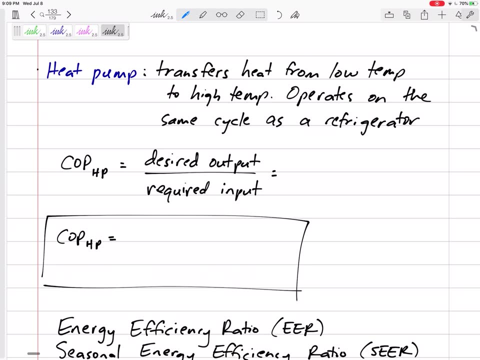 generating, you know, work from, from nowhere. Um, the coefficient of performance could be greater than one. All right, A heat pump is a refrigerator. Okay, A heat pump is a refrigerator. It does the same thing: It transfers heat from low temperature to high. 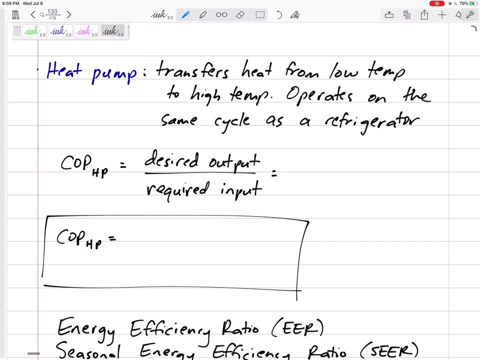 temperature? Uh, it's the same cycle as a refrigerator. Uh, it's just that it's almost as if we put a refrigerator in the window and the refrigerated space is the outside air And instead of spitting it out- the back, you know- towards the wall behind our refrigerator, it just 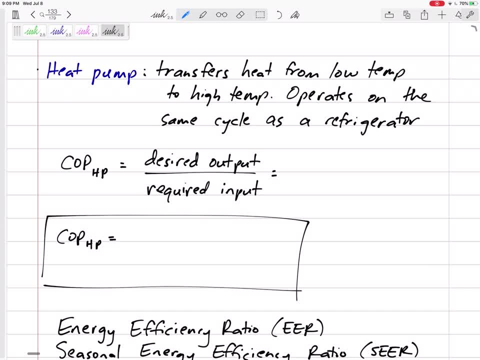 a heat pump spits it into our room. A heat pump heats up our room even though the room has a higher temperature than outside. All right, Does that make sense? Right, Yeah, If, if it's cold outside and warm. 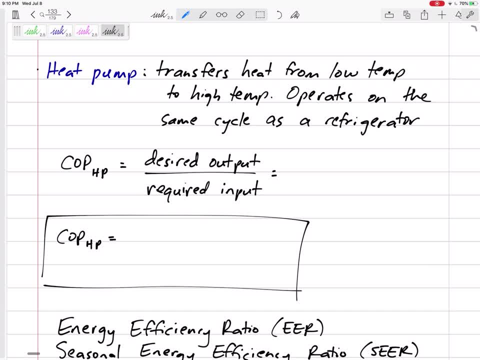 inside um and we want to heat up or keep our space heated um, we can't let the cold air come in. but if we could get some of the cue from the cold air and put it into the uh room, then 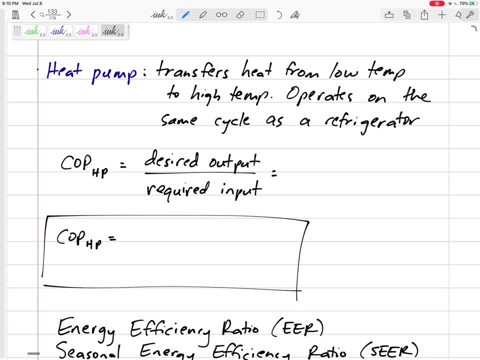 uh, that's, that's what we're. that's what we're, that's what we're doing, All right, Okay, So for a heat pump, what are we really desiring? We're really desiring the QH, as much QH as we can. 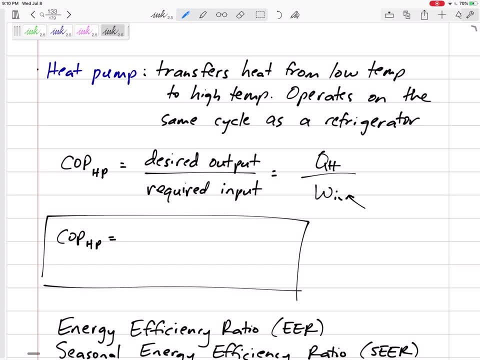 uh divided by the work in or the net work in. This is QH minus QL. Okay, The coefficient of performance of a heat pump is QH over QH minus QL, or one over one minus QH over QH. So a little bit different coefficients of performance for a heat pump versus the. 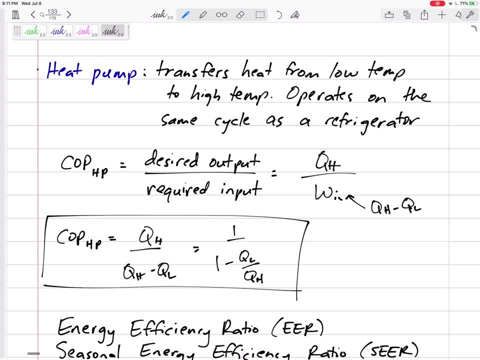 coefficient of performance for a refrigerator. but we have coefficients of performance so that we can compare one refrigerator to another, uh, so that we can compare, um, which one is better, uh, which one is more desirable Uh. the coefficient of performance of a heat pump is: 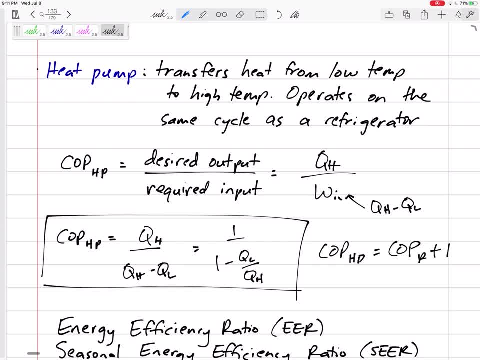 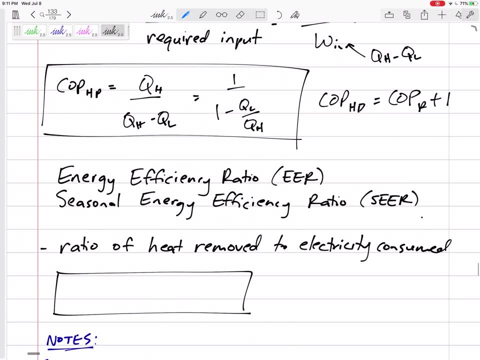 equal to, mathematically, the coefficient. it's one more than the coefficient of performance of the refrigerator. Okay, All right, Real, briefly, some definitions. We have energy efficiency ratio, or the seasonal energy efficiency ratio. uh, and it is the ratio of heat removed to electricity consumed. Um, 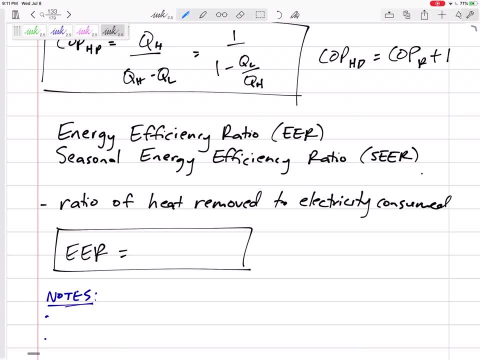 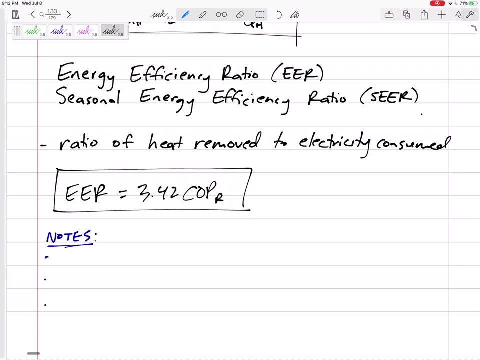 I don't have much uh notes on this, except that the energy efficiency ratio is 3.14, or 3.412, times the coefficient of performance of the refrigerator. Um, we're not going to use that and I don't have much many details about that. Uh, but a few notes. a few notes on these. 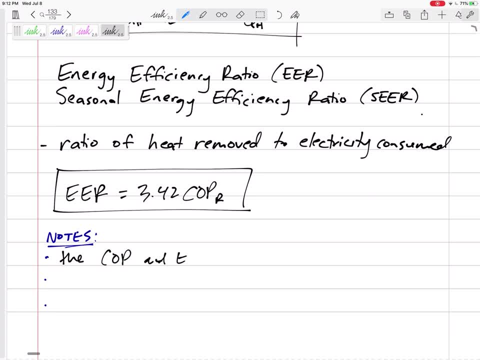 The coefficient of performance and the energy efficiency ratio decrease with decreasing temperature. Okay, What does that mean? What does that mean? That means, uh, it takes more energy to keep our fridge very cold. right, If we want to keep our fridge very cold at a lower temperature. 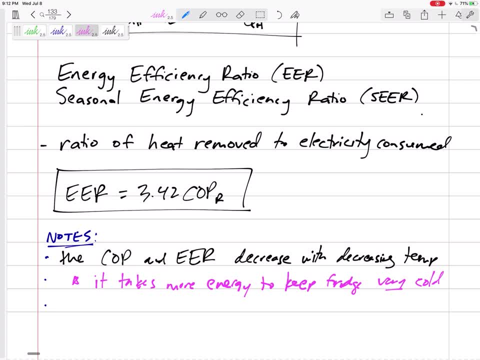 it's going to not have as good of a coefficient of performance. It's not going to be doing as good. It takes more energy to keep our fridge very cold. So if we want to keep our fridge very cold, at a lower temperature.